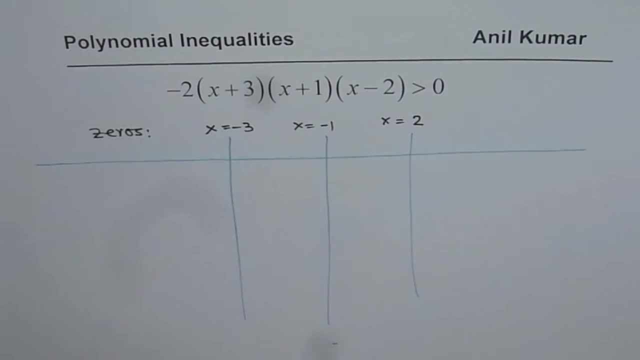 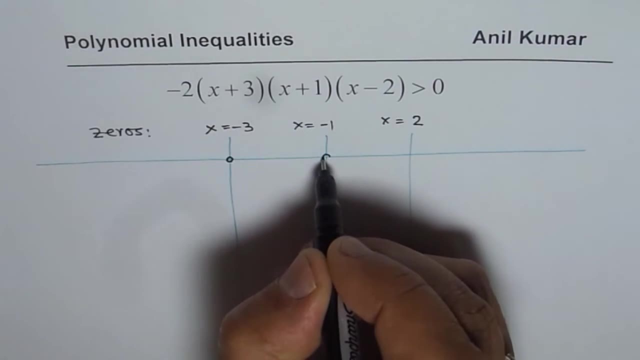 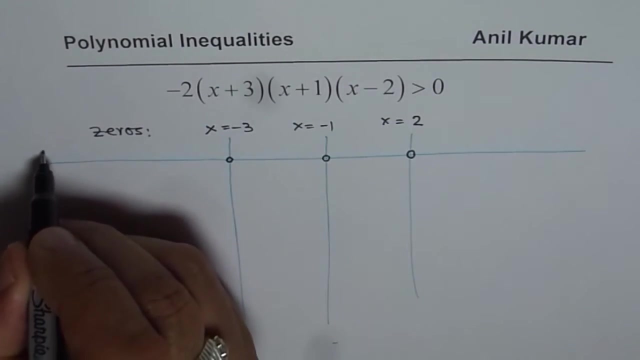 that these are, let us say, zeros, right? So on the x? y plane, if I have these zeros here, let's say these are my zeros, then the x? y plane is divided into 4 different intervals, right? So let me write down the. 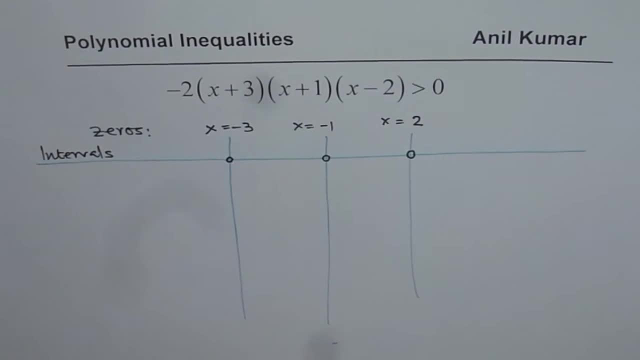 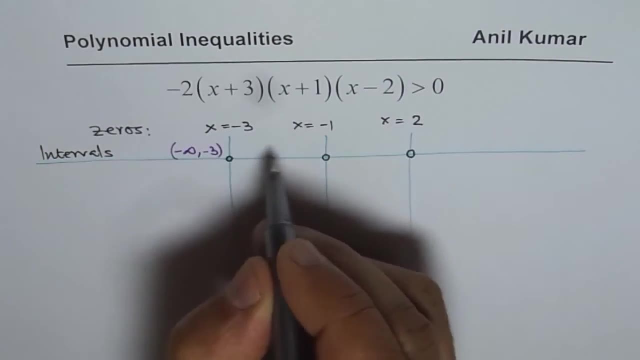 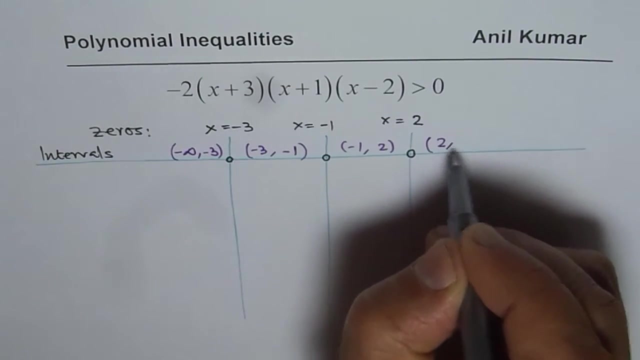 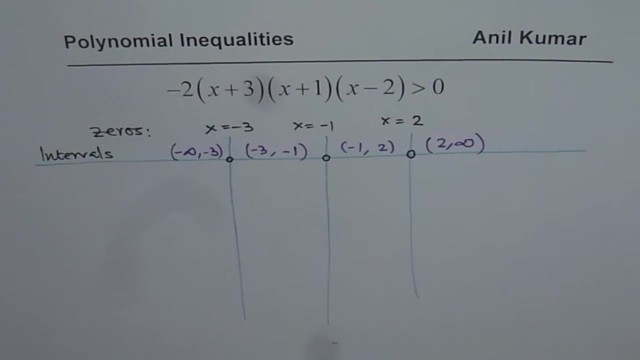 intervals here. So if you see, from left to right this interval is from minus infinity to minus 3, then we have from minus 3 to minus 1, and then from minus 1 to 2, and from 2 to infinity. So 3 zeros means 4 intervals. Now the question is that during these 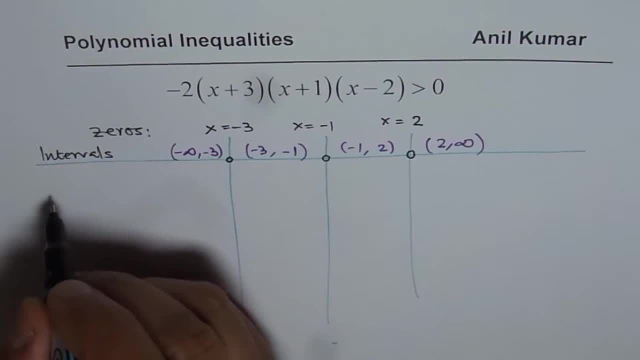 intervals, the sign of the function always remains same, right, It only changes at zeros. That is the concept. So what we can do is we can take some test points. So we'll take test points in the given intervals and see whether the function is. 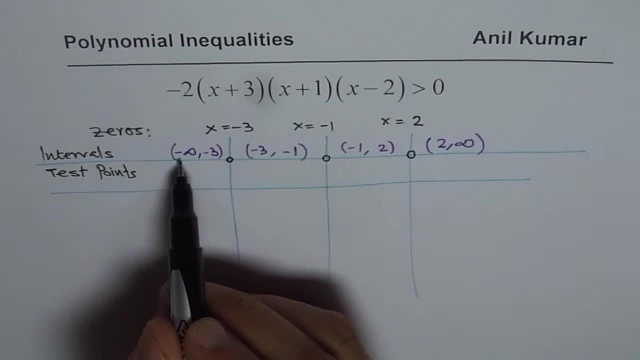 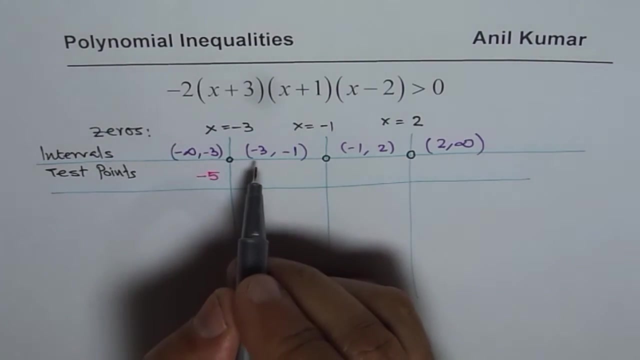 positive or negative. A test point in this interval minus infinity to minus 3, could be minus 4, minus 5.. Let us write down in a different ink. Let us write down this interval as minus 5.. In this interval, a test point as minus 5.. A test point- x value- we mean between minus 3 and minus 1- could. 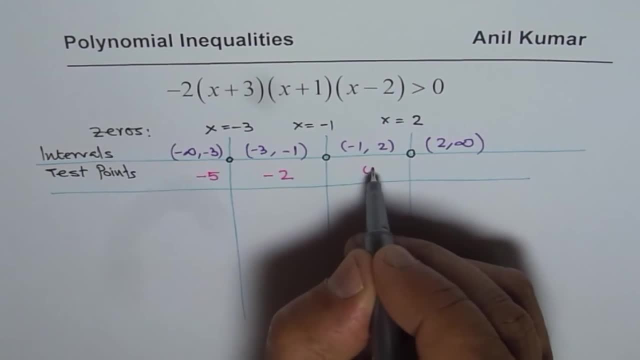 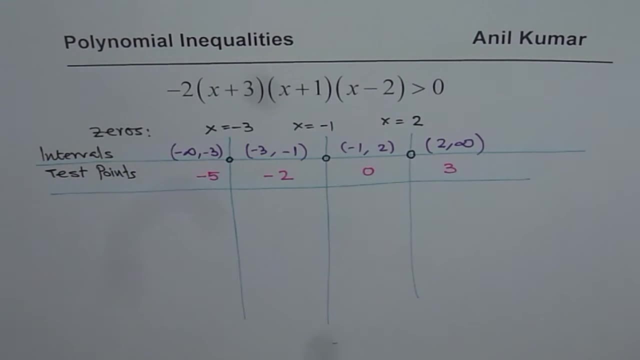 be minus 2.. Between minus 1 and 2, 0 is a good test point. 2 to infinity. let us take 3 as our test point, So you could take any point in that interval. Now what do we need to test? We will. 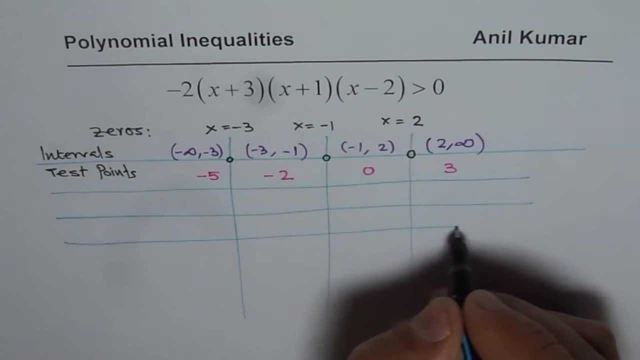 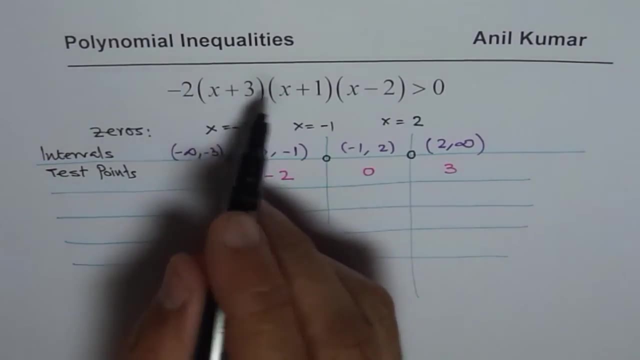 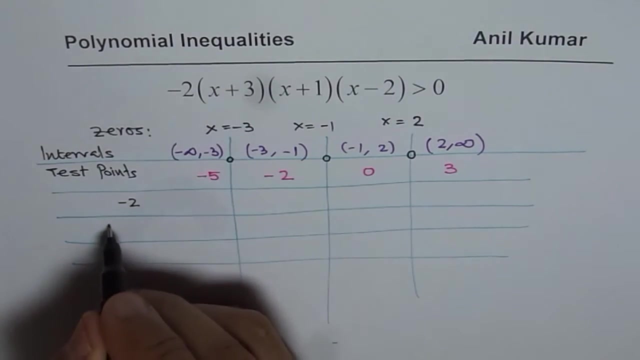 test each factor whether it is positive or negative. So that is the whole idea. So we will test each factor. So let us write down these factors one by one. Well, minus 2 is our first factor. So let me write down the factor minus 2 first, and then we have x plus 3, and then we have 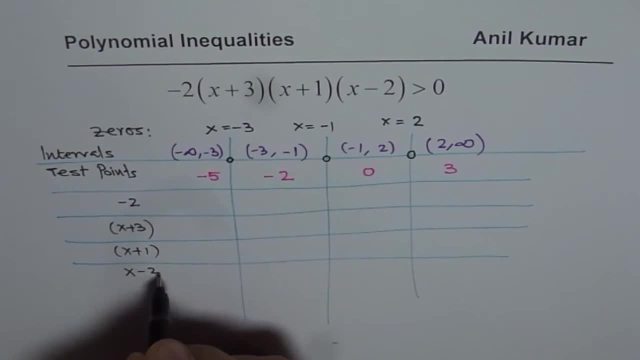 x plus 1, and then we have x plus 2.. x minus 2.. So these are the four factors for us. Now, as you know, minus 2, whether x value is minus or positive, it will remain negative 2.. Now, while we are testing, we 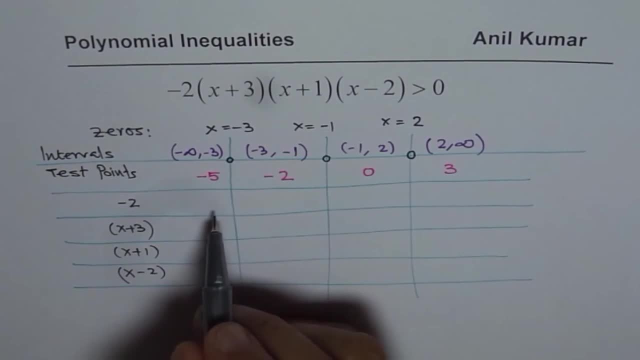 are actually interested only in the sign, not in the value. So sign for minus 2 will be negative in each interval. correct Now: x plus 3.. If I substitute minus 5 here it becomes minus 2, negative sign. If I substitute negative 2 here, it becomes plus 1, sign is: 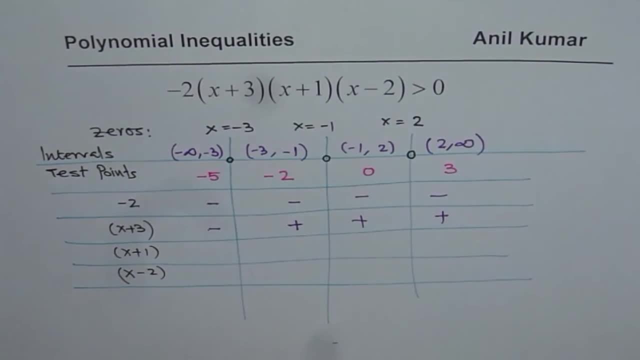 positive. 0 and 3 will also give us positive signs: x plus 1.. Substituting minus 5 gives us minus 4, negative sign. Minus 2 plus 1 is also negative. 0 plus 1 is positive 3. 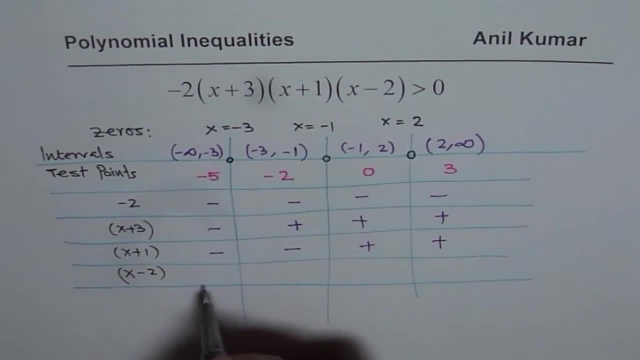 plus 1 is positive, x minus 2.. When x is minus 5, it is negative. When minus 2, it is negative. For 0, again it is negative, And then for 3, it is positive. So that is how each factor is within these intervals. 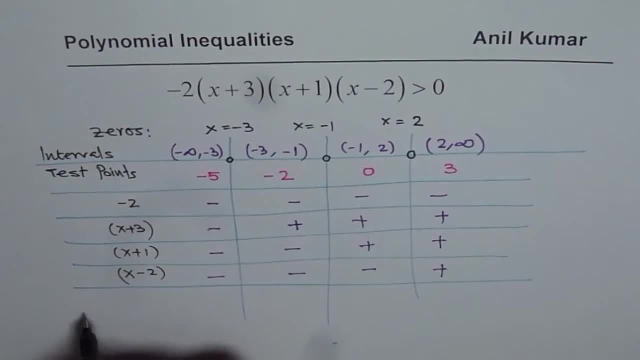 Now, within these intervals, how will the function be? Now, what is function? Function is product of all this right. So our function here is: minus 2 times x plus 3 times x plus 1.. 1 times x minus 2.. Now how can you tell me how will the sign change? So let's write. 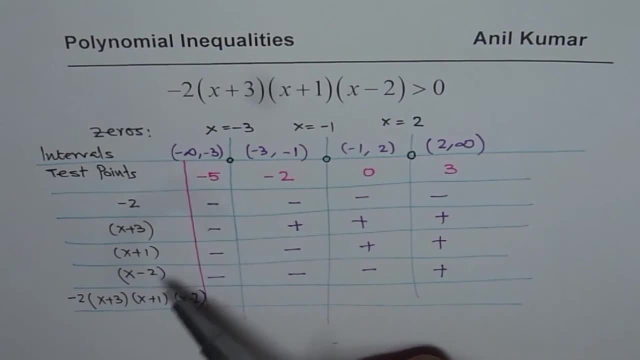 from left to right. If we multiply these four factors, that means negative four signs. even number of negative signs, when multiplied, will give us positive. right Odd number will give us negative. Even number will give us positive Odd number will give us negative. When we 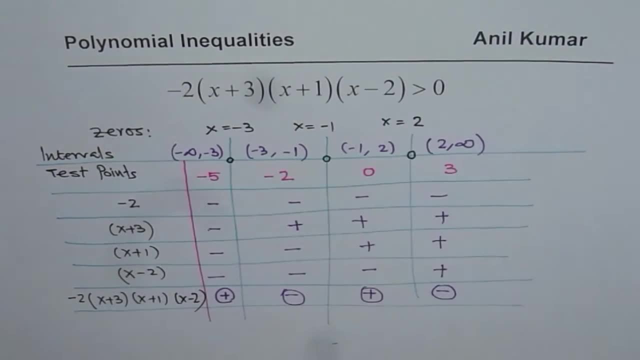 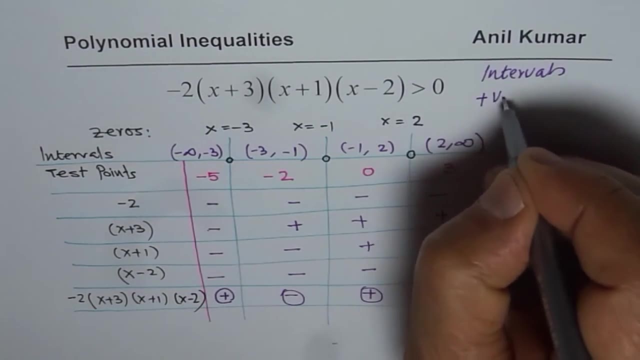 see that this is positive, we will see that this is negative. We will see that this is positive When we see that this polynomial is greater than 0,. what are we looking for? We are looking for intervals where the function is positive. Is that okay? So we get our. 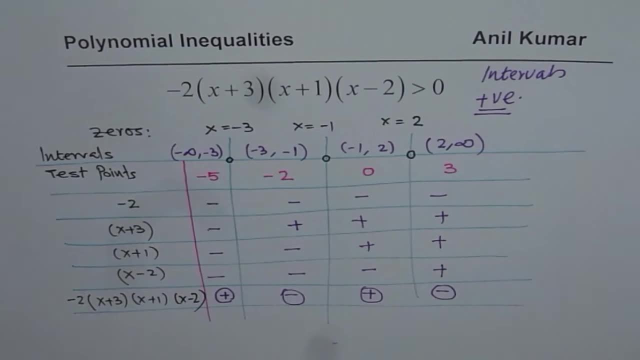 answer: The function is positive in these two intervals. correct Means these two intervals And therefore that is our answer. right? So therefore that is our answer. We can write down our answer as Minus infinity to minus 3 and from minus 1 to 2, right. At times we prefer to write. 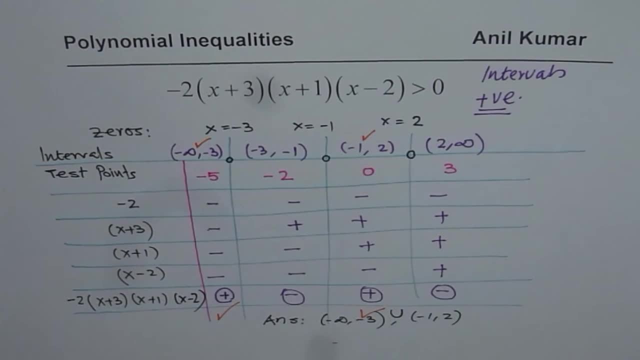 union sign also correct. So that becomes the solution for the given question. Now, as I said in the very beginning, we will test with the help of a sketch. Minus means this. minus means the leading coefficient is negative. right side is down. right Right side is down.